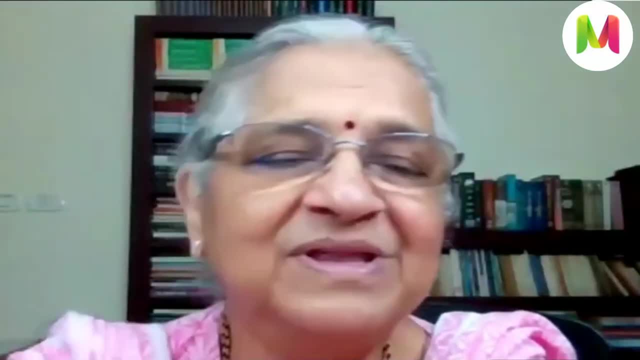 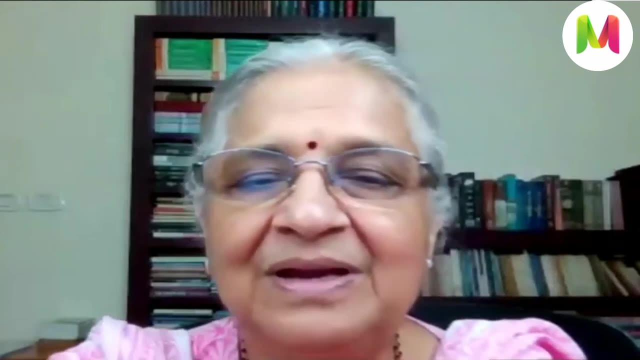 Including husband and everybody and in-laws. they say: because mother was working, the child did not do well. They never said father was working, the child did not do well. Nobody says It's only mother, And mothers also feel I wish I could have spent more time. This is all myth. 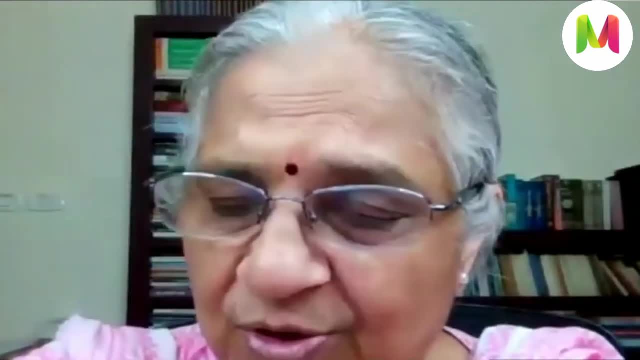 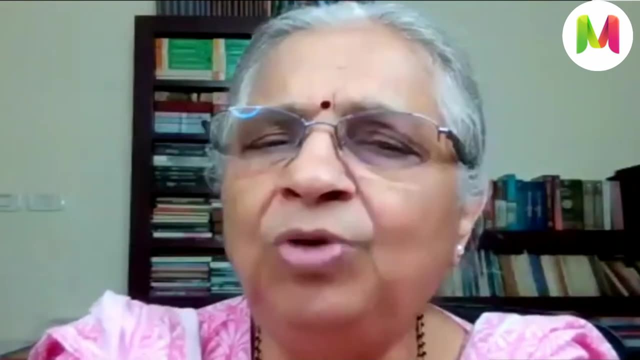 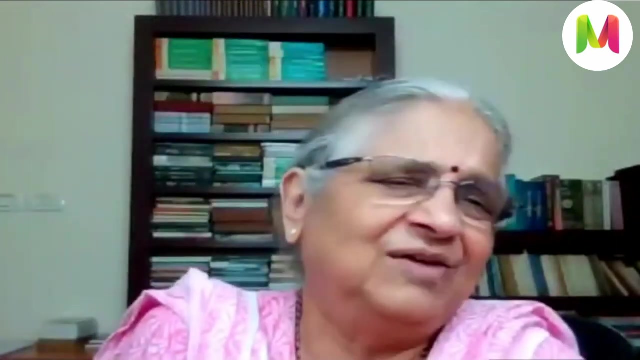 If you want to spend time with your child and you want to work also, you require a great support, which I have talked. Then for you also, I will tell you you have to spend all weekends with your child. No party, no socializing. I did that. I will never attend a wedding or party. I will go with my child. 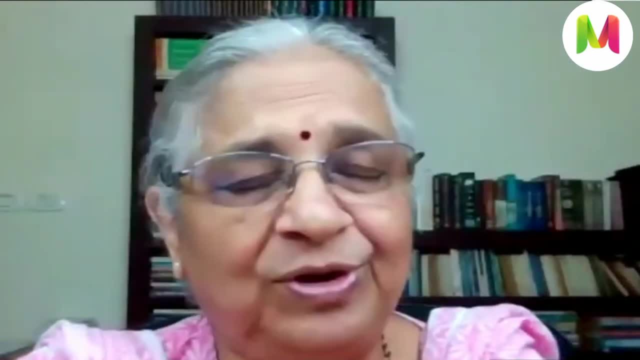 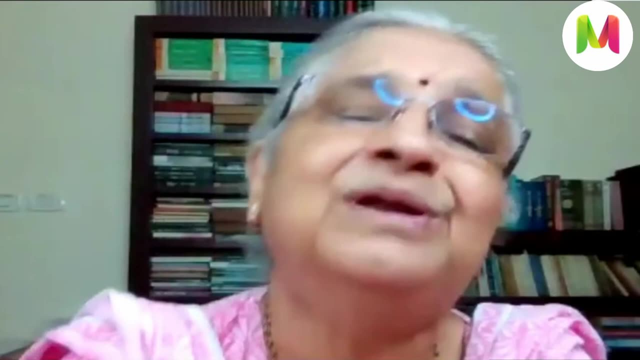 What a child will enjoy, I will do, rather than what I will enjoy. The child enjoys zoo go. The child enjoys the park go. The child wants to play hide and seek play. Okay, with respect of your age, The child wants you should read a story read. 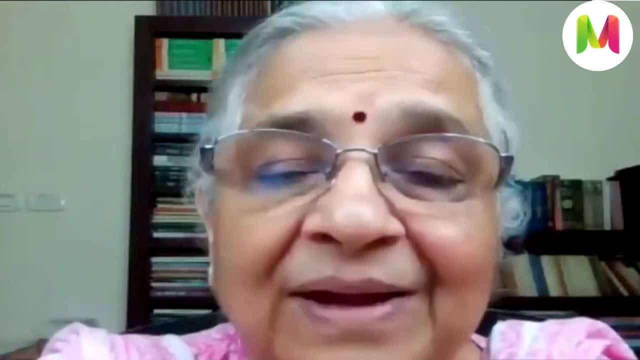 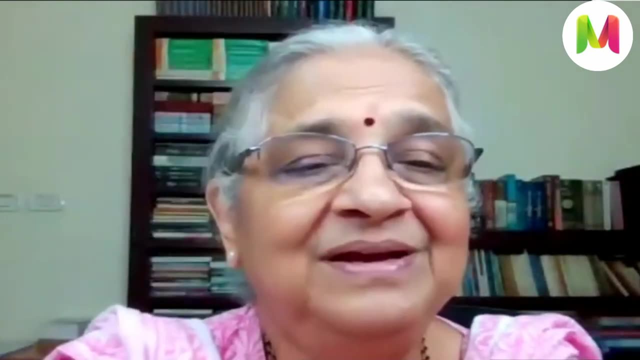 Engage yourself with the child whenever you have time And I used to explain when they were big. you know better. Amma is working and you should cooperate. So when you know I, you know. my time was different also When they used to go to school. I used to teach. 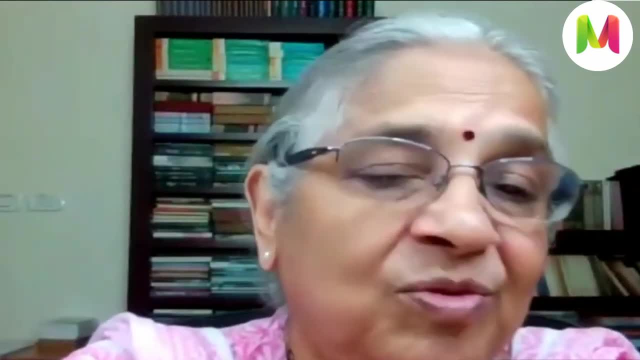 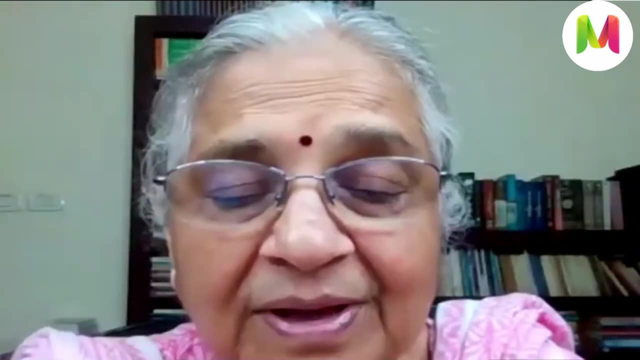 Before they come back, I will come back. We didn't. we did not have work from home in those days. There was no baby crush or baby care. Nothing was there. So make your life a priority, with the child, along with your work. 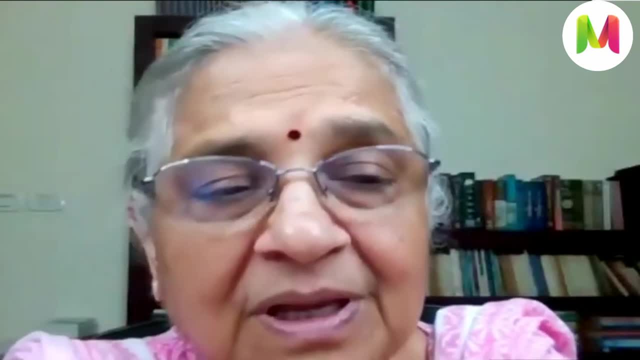 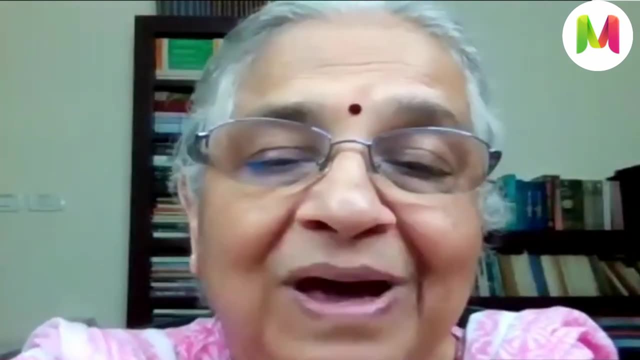 Okay. you sleep with the child as early as possible. You sleep with the child or before the child gets ready. You have to do all these things then only it is possible to balance. That means next 14 years. you are the best friend of your child. 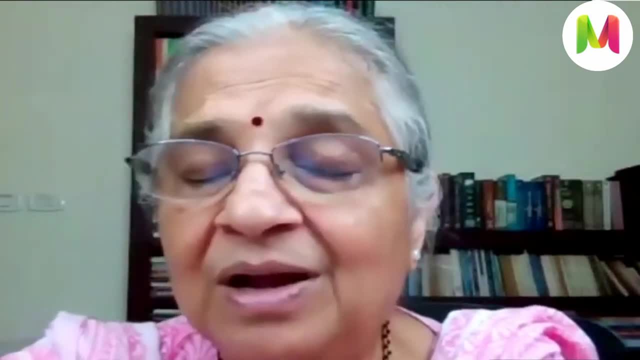 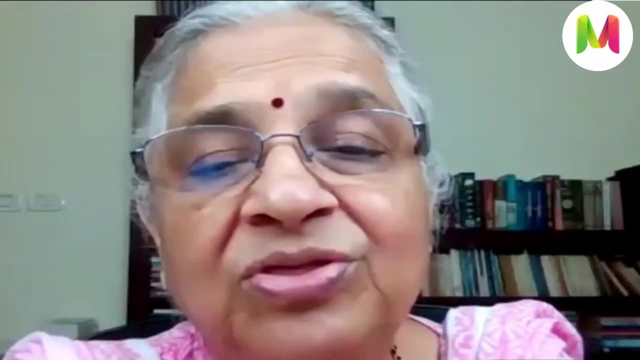 And you should tell your child: look and build a confidence with your child. When the child makes a mistake, he or she comes back and tells: Amma, I made a mistake. Not third person comes and tells you. I always told my children when you make a mistake. 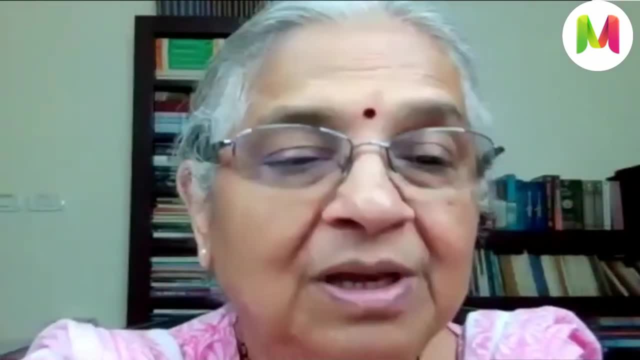 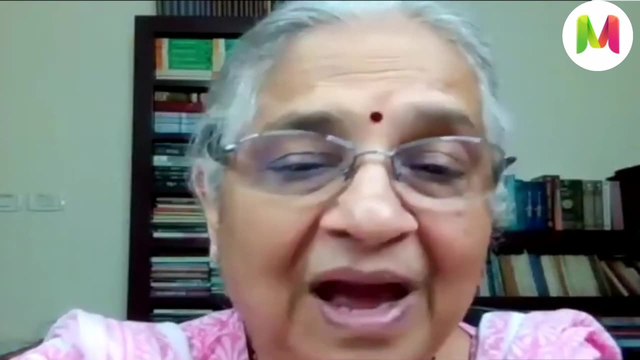 However good or bad, mistakes are bad. only Come and tell me and I will tell you how to improve, how to correct what is wrong. Then I want to know my child, only the true child, not with somebody else. Okay,